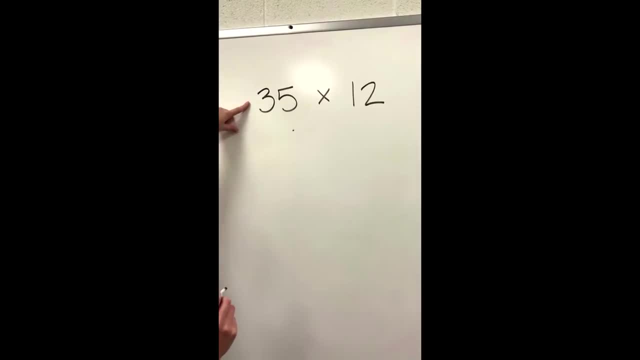 So first thing is we have our multiplication problem: 35 times 12.. The first thing we need to do after that is expand these two numbers. We need to break it down into its tens and its ones. I've got three tens. I've got three tens, which is 30, and five ones. So that is 30 plus five. 12 is one ten plus two ones. Okay, so that's step one. The next step would be to draw a large box. 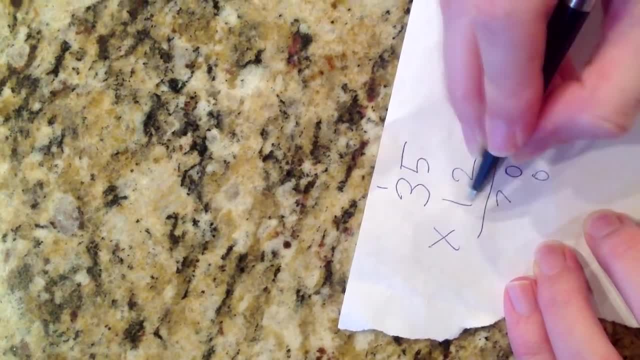 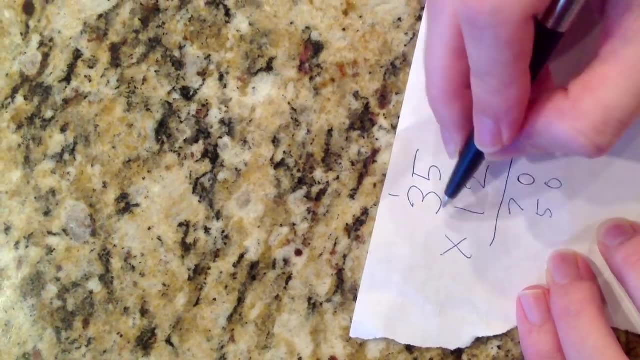 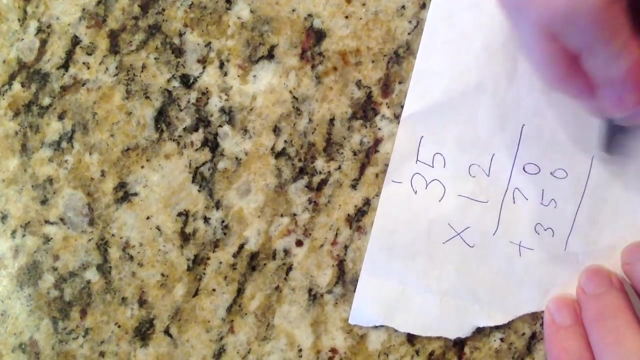 And then for the next number we add a zero, And then it's five times one, And then again, because it's not above 10, there's no number to carry- Then it's three times one, which is three. So now we add 70 plus 350, which gives us 420. 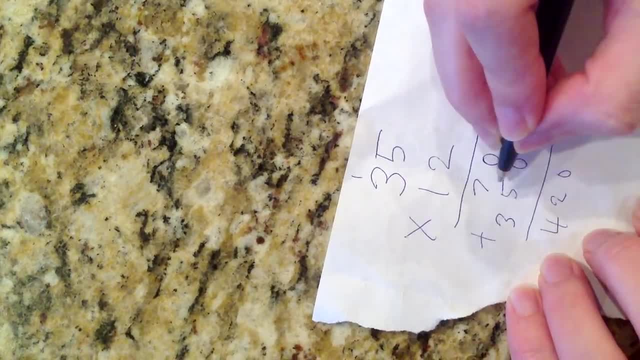 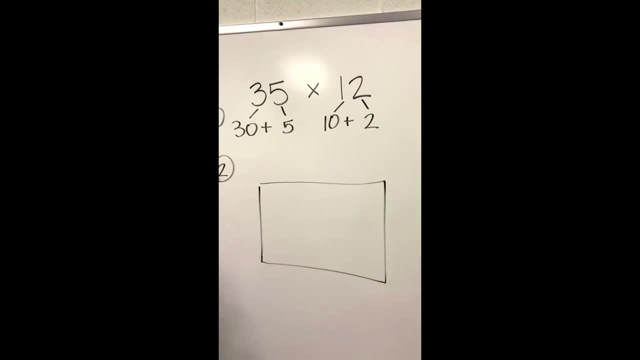 So, and the way you do that? obviously, zero plus zero is zero, Seven plus five is 12.. Carry the one And that's how we get the four in that column. Okay, and on this box we're going to put both of our expressions. 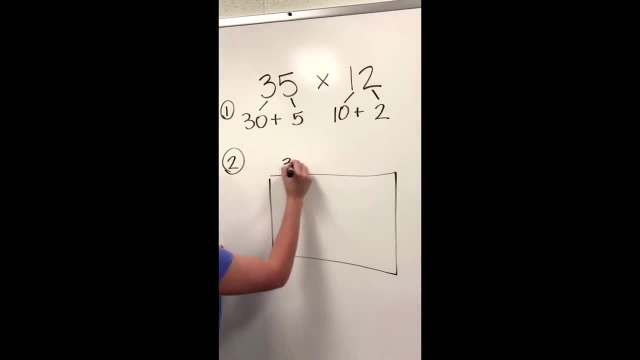 We're going to put our expanded numbers. So on the top I'm going to put 30 plus five And on the side I'm going to put 10 plus two, Where your plus signs are. I want you to draw lines through the middle and down it. 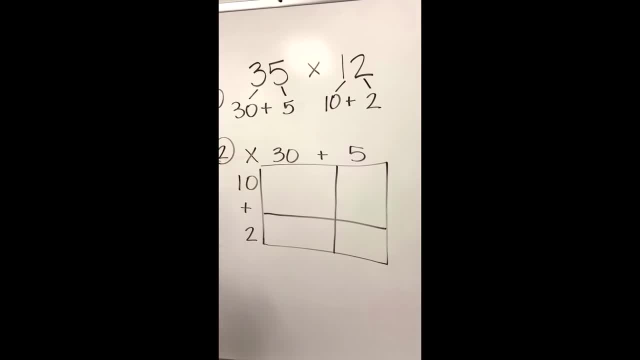 And then in the very corner, we're still multiplying. so I'm going to put a big multiplication sign, Starting with our very first number. on the top we say 10 times this, 10 times that. So first we're going to do 10 times 30.. 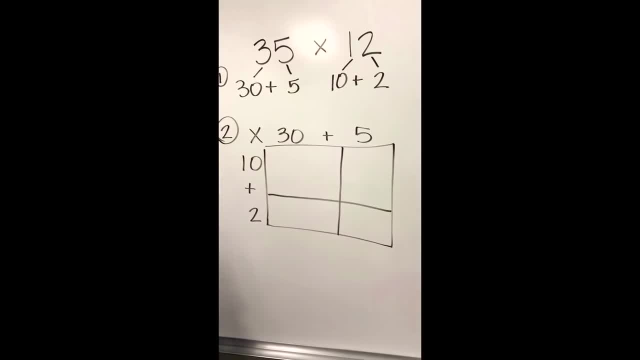 Sometimes it gets a little tricky when we have those extra zeros on there, when we're multiplying by a 10. So I like to say: one times three is three, And how many zeros do we have? We've got two, so we attach them to the end of the number. 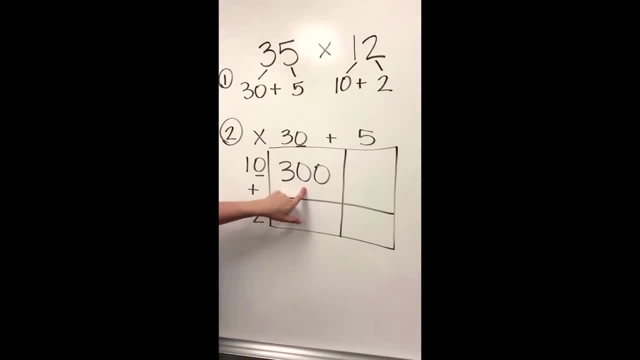 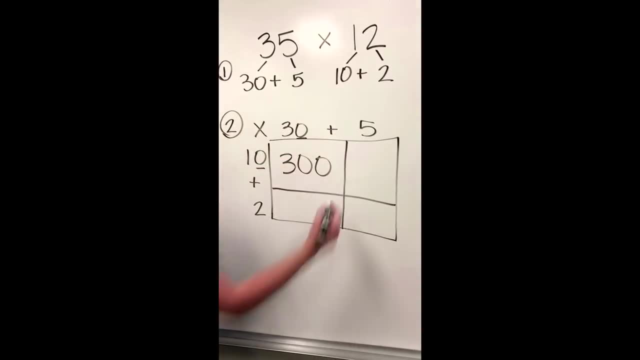 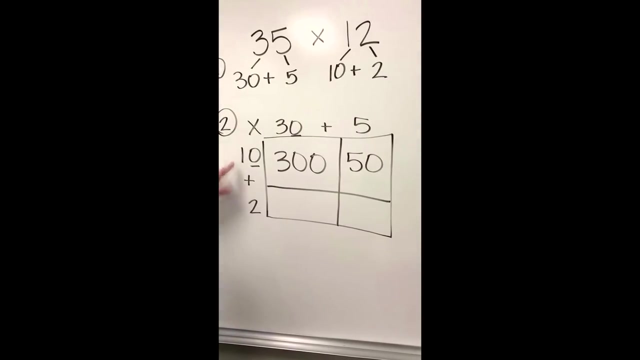 So 10 times 30 is 300.. We did 10 times 30.. 10 times this, 10 times that, 10 times five is 50, so it goes in the first box And then we do two. We go down to the two because we're done with the 10..